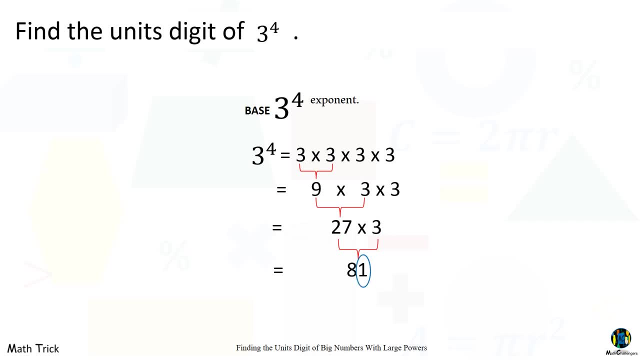 To find the unit's digit of numbers with small powers is easy, but what if you have a big number with a small power? What if you are asked to find the unit's digit of large powers, like 4 raised to 77th power? 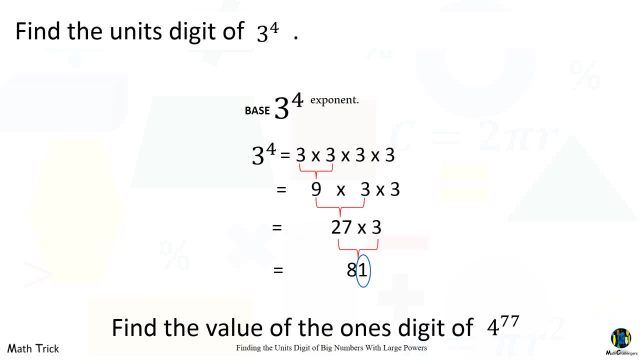 How are you going to answer it right away? Since raising to a power is repeated multiplication, we can find your unit's digit with a simple multiplication pattern. even when you're working with large powers, The best way to do it is to observe how the one's digit changes with each multiplication. 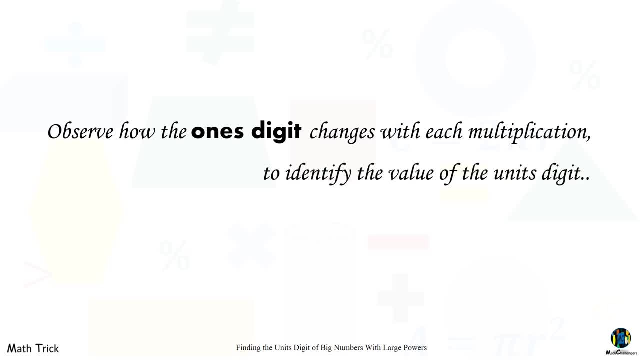 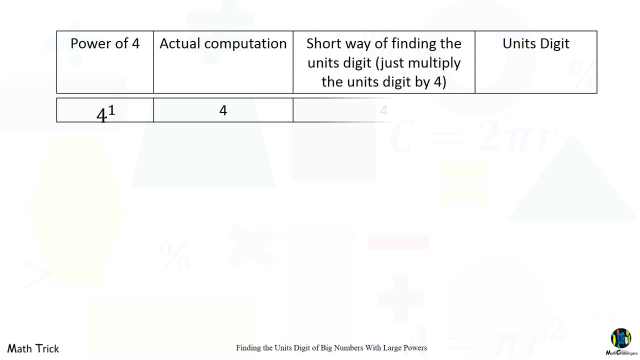 to identify the value of one's digit. Let's take a look at the powers of 4.. 4 raised to 1 is 4,, so the unit's digit is 4.. 4 raised to 2nd power is 16, so the unit's digit is 6.. 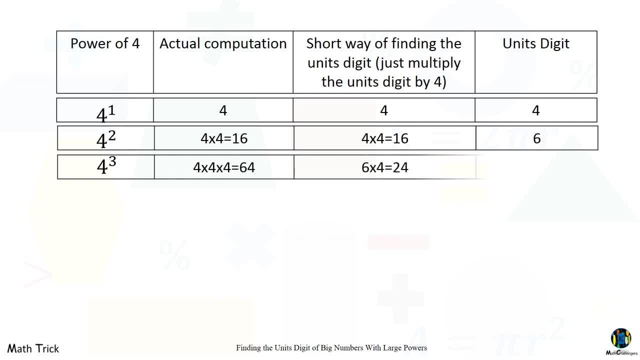 4 raised to 3rd power is 64, so the unit's digit is 4.. 4 raised to the 4th power is 256, so the unit's digit is 6.. If we continue raising the power of 4, the same pattern continues. 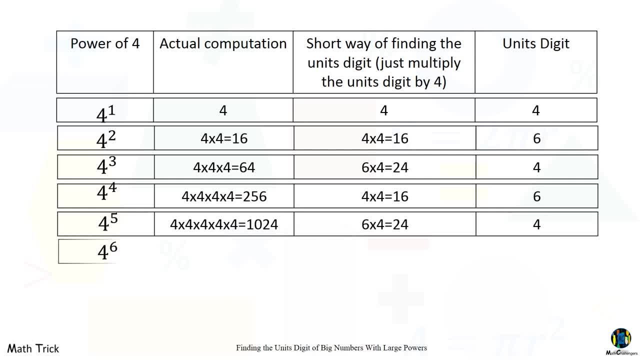 the one's digit will be 4 and 6.. Notice that when 4 is multiplied every time with its own self, the last digit changes On the 3rd multiplication. 4 raised to 3rd power has the same unit digit as 4 raised to 1.. 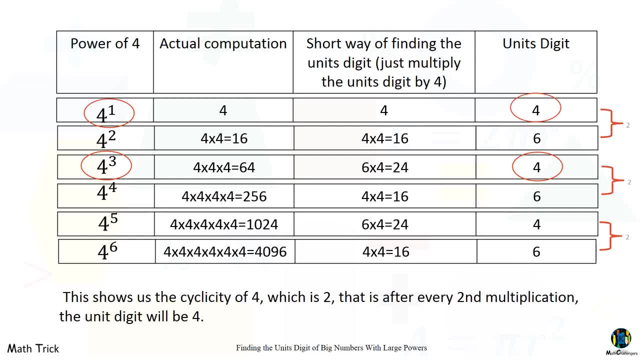 This shows us the cyclicity of 4, which is 2.. That is, after every second multiplication, the unit digit will be 4.. The cyclicity of any number is about the last digit and how they appear in a certain defined manner. 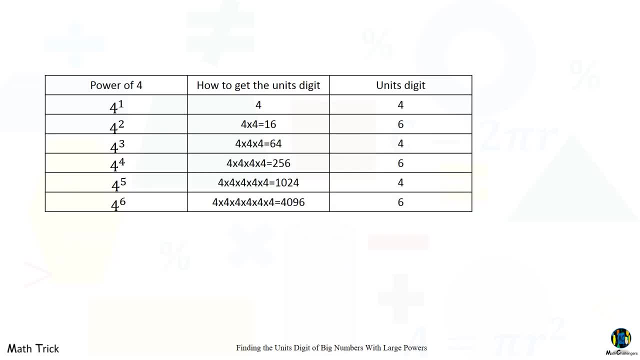 Now let us use this concept of cyclicity to calculate the unit digit of a number. So define: for the unit's digit of 4 raised to 77th, power, divide the exponent by 2.. 77 divided by 2 is 38, remainder 1.. 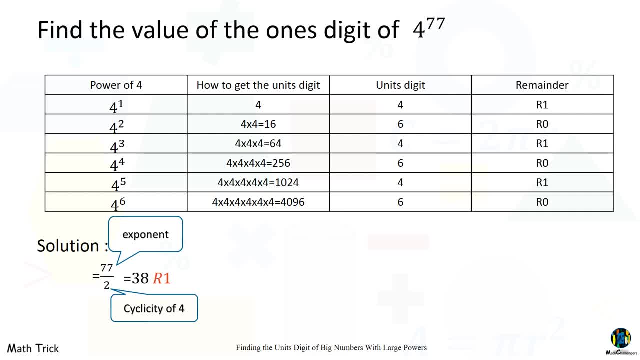 Since there are only two possible unit's digit in a power of 4.. If, after dividing the exponent by 2, the remainder is 1, then the unit's digit will be 4.. If there is no remainder, on the other hand, the unit's digit will be 6.. 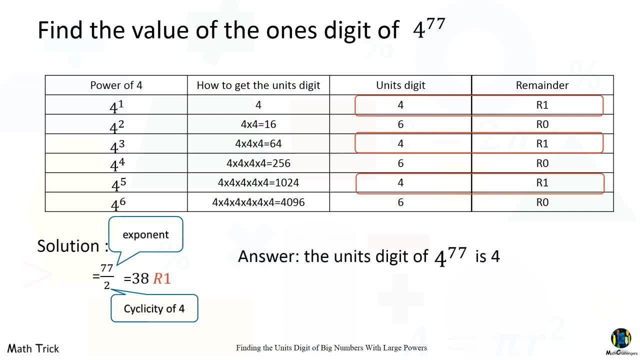 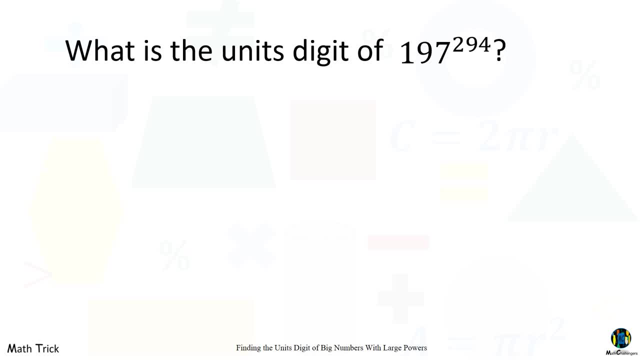 The unit's digit, therefore, of 4 raised to 77th power is 4.. What is the unit's digit of 197 raised to the power of 294?? What is the unit's digit of 6 raised to the power of 97?? 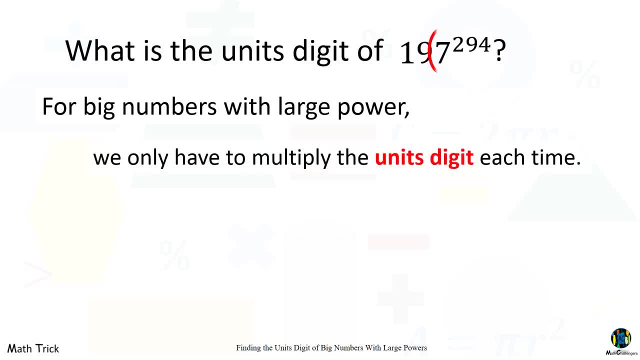 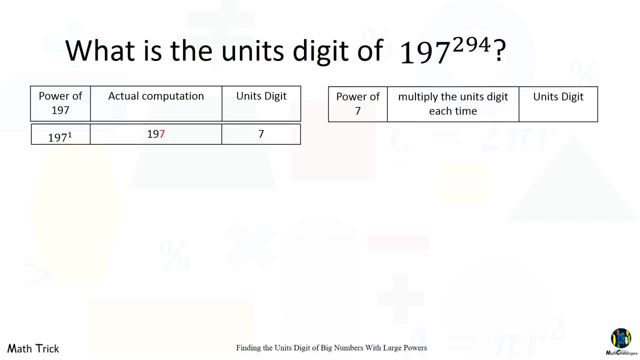 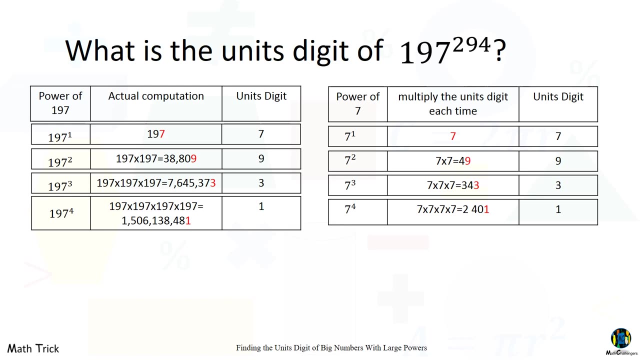 For big numbers with large power, we only have to multiply the unit's digit each time. Observe the examples below: What is the unit's digit of 7 raised to the power of 997?? The unit's digit of 197 squared is the same as the unit's digit of 7 squared. 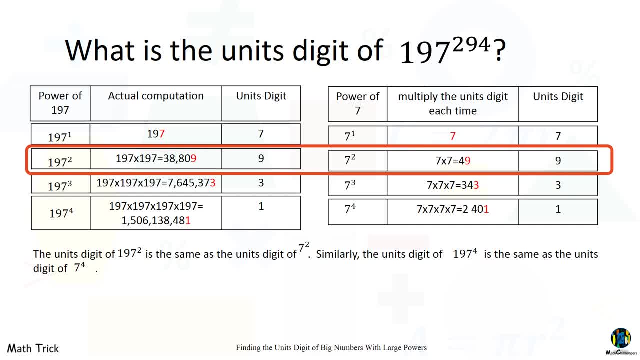 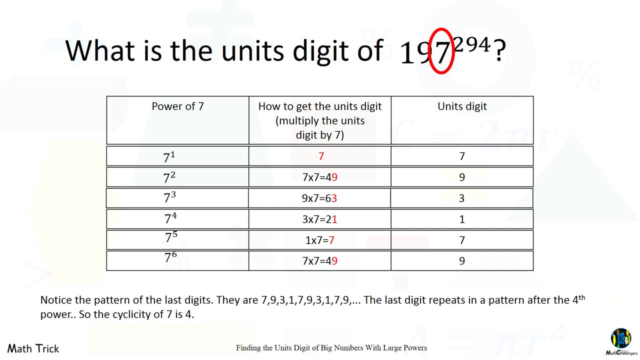 Similarly, the unit's digit of 197, said infinite number, to the 4th power is the same as the unit's digit of 7 to the 4th power. Notice the pattern of the last digits. They are 7,, 9,, 3, 1, 7, 9,, 3, 1,, 7, 9.. The last 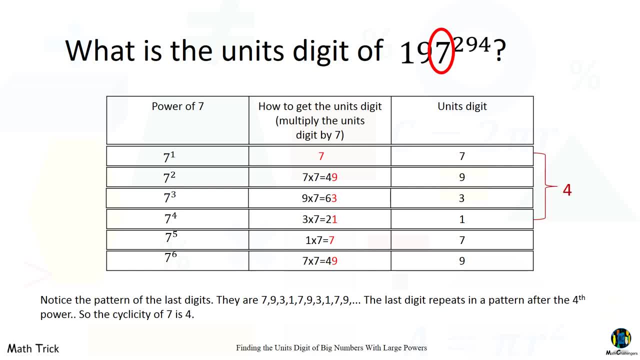 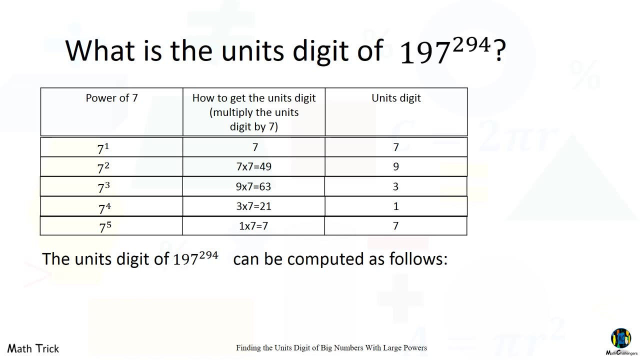 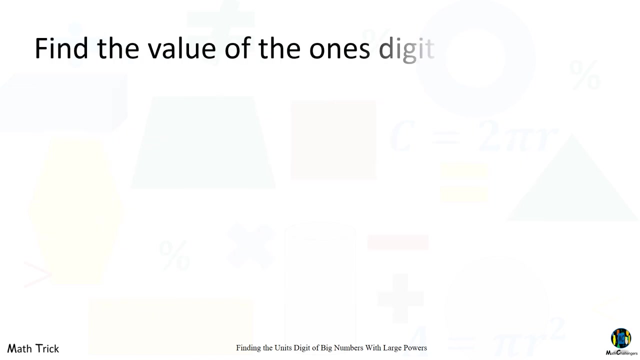 digit repeats in a pattern after the 4th power, So the cyclicity of 7 is 4.. The unit's digit of 197 raised to the power of 294 can be computed as follows: Find the value of the 1's digit of the 33 raised to 303 power. 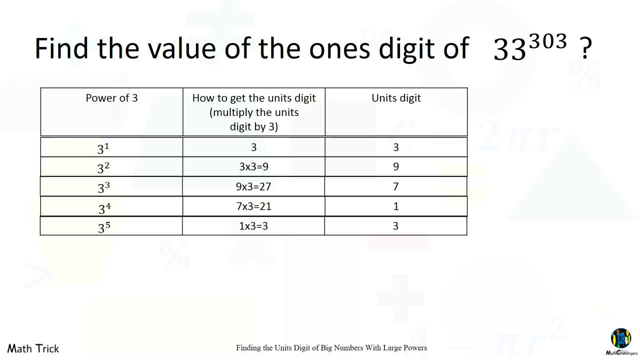 Upon examining the unit's digit of the powers of 3,, we can see that the cyclicity of 3 is 4.. If you complete the table for 303 rows, how many times will this pattern repeat? 303 divided by 4 is 75, with a remainder of 3.. 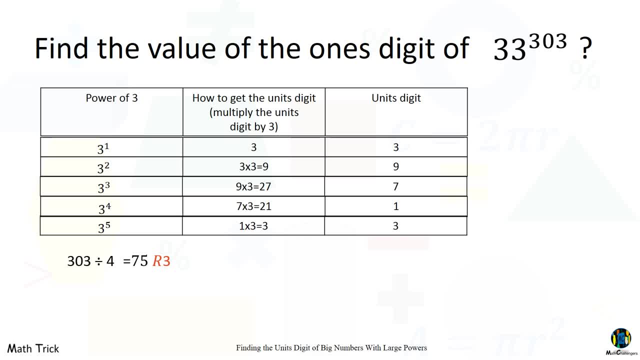 So the pattern will repeat 75 times, and then there are 3 more rows. The unit's digit of 33 raised to the power of 294 can be computed as follows: 303 raised to the power of 294 is 7.. Here's a better trick. 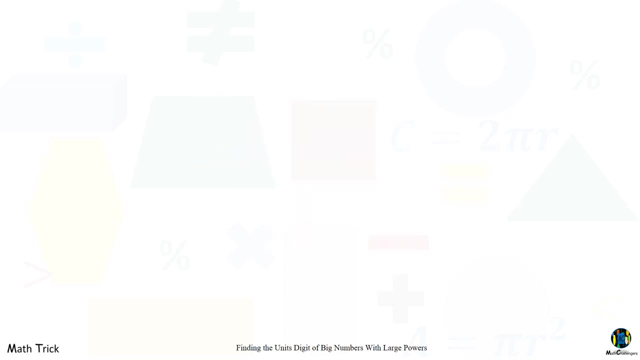 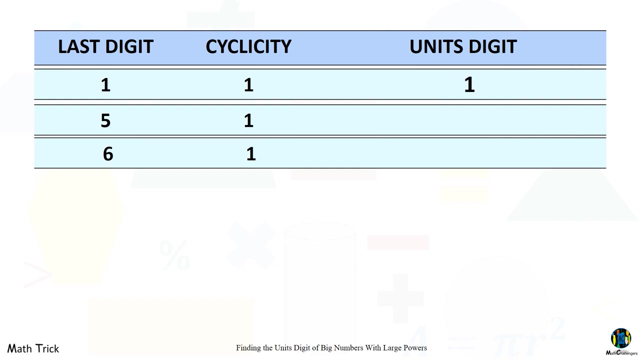 To find the unit's digit of a number, regardless of how big it is, just identify the last digit, Then determine its cyclicity. For numbers with 1, 5 and 6 as their unit's digits, the cyclicity is 1.. And the unit's digit is always 1, 5 and 6 respectively. Examples: 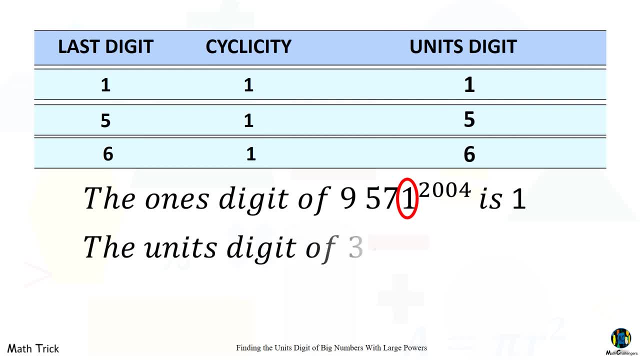 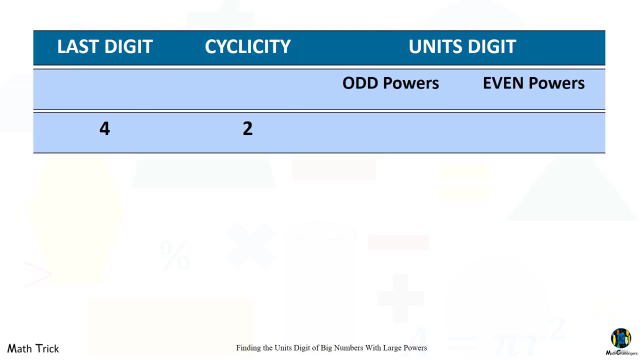 For numbers ending in 4 and 9.. The cyclicity is 2.. The exponents can either even or odd For numbers ending in 4,. if the exponent is an odd number, the unit's digit is 4.. If the exponent is an even number, the unit's digit is 6.. 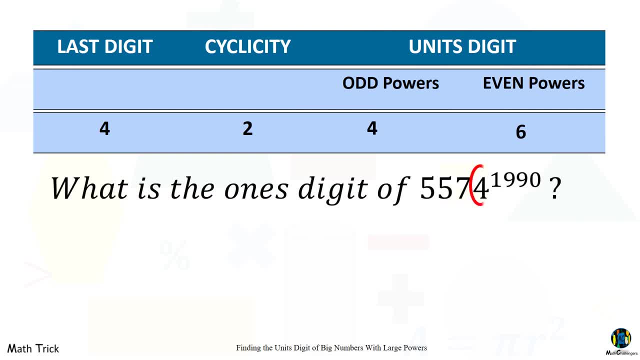 Examples: What is the 1's digit of 5,574 to 1,990th power? Find the unit's digit of 7,854 to the 2,467 power. To answer these questions, you only have to look at the exponents. 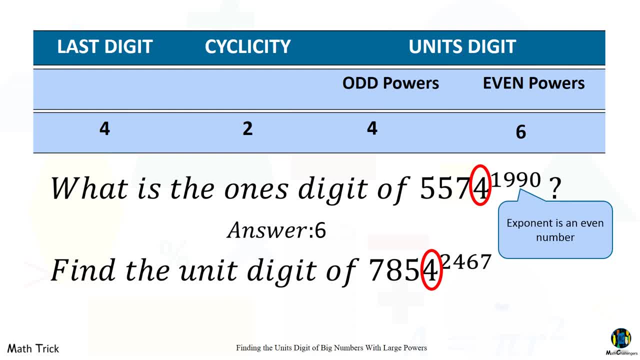 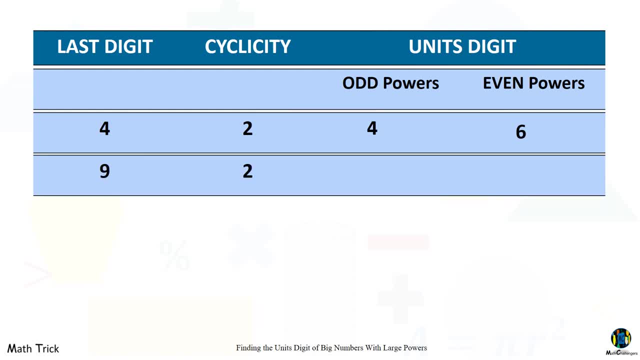 If it is an even number, the unit's digit is 6.. If the exponent is an odd number, the unit's digit is 4.. For numbers ending in 9,: if the exponent is an odd number, the unit's digit is 4.. 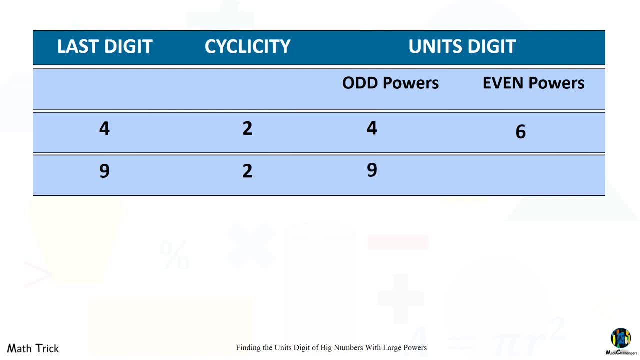 The unit's digit is 9.. If the exponent is an even number, the unit's digit is 1.. What is the 1's digit of 2,359 to the power of 100?? Find the unit's digit of 6,549 to the power of 691.. 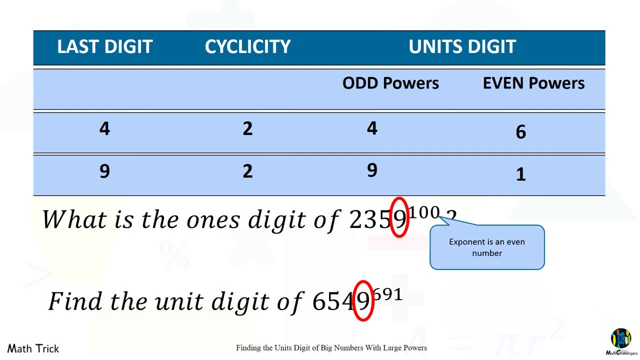 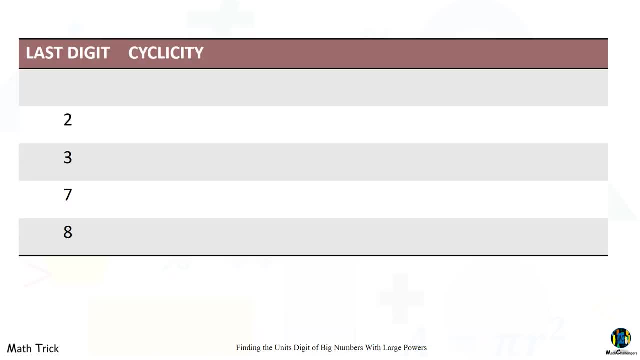 If the exponent is an even number, the unit's digit is 1.. If the exponent is an odd number, the unit's digit is 9.. For big numbers ending in 2,, 3,, 7 and 8 with large powers, the cyclicity is 4.. 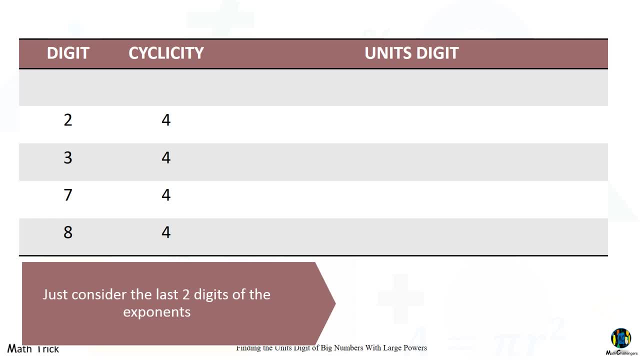 For mental calculation, just consider the last two digits of the exponents, Then apply the divisibility rule for number 4.. If the last two digits are both 0, or if the last two digits are divisible by 4,, these are the last digits. 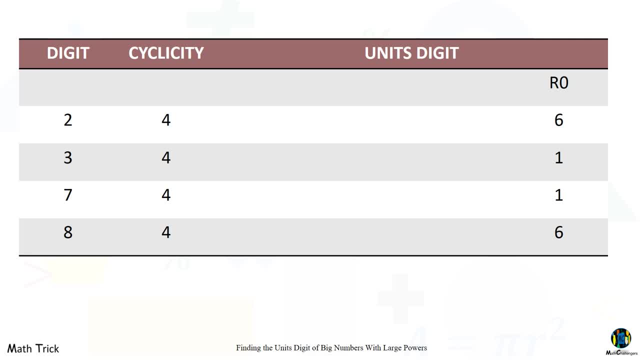 If there is a remainder, then the unit's digit can be the following: If the last two digits are both 0, or if the last two digits are divisible by 4,, these are the last digits. For example, what is the unit's digit of 343 to the 155th power? 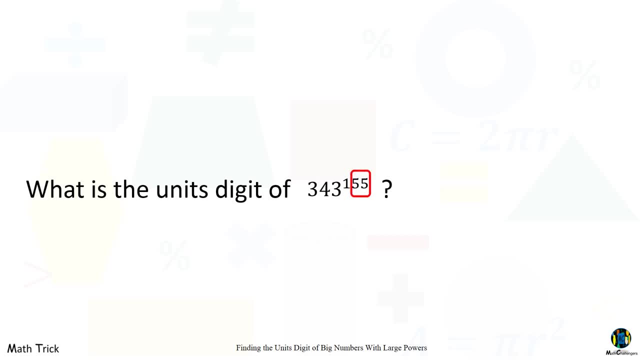 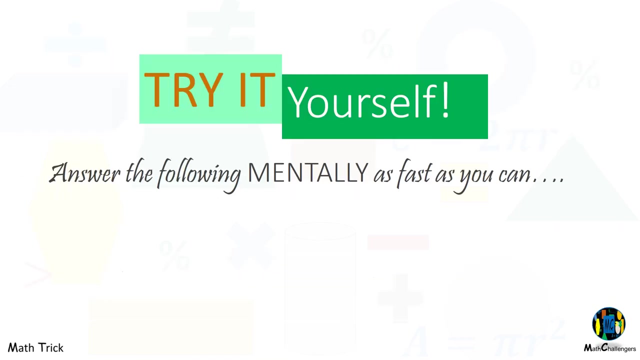 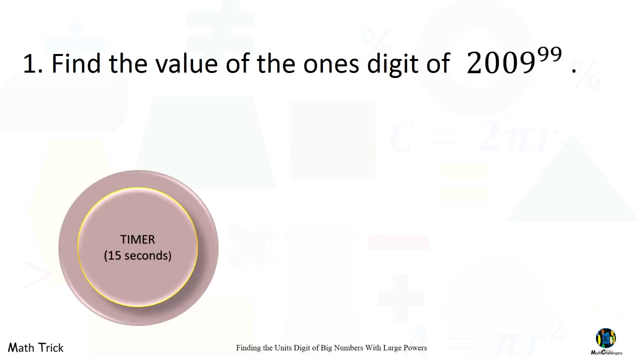 The last two digits in the exponent is 55.. 55 divided by 4 is 13, remainder 3.. The unit's digit of 343 to the 155th power is 7.. 1. Find the value of the 1's digit of 2009 raised to 99th power. 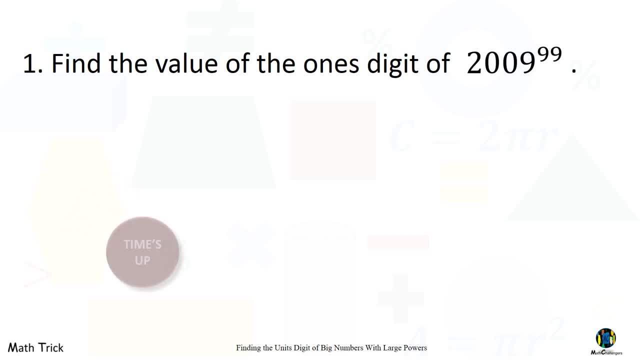 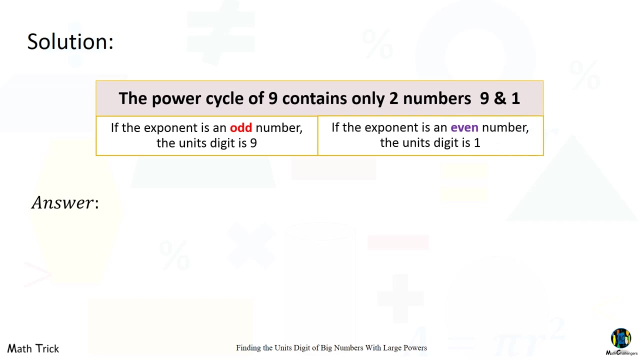 2. What is the unit's digit of 167 raised to 35?? 2. What is the unit's digit of 167 raised to 26?? the upper left second digit during the calculation, the upper left second bebcle and the upper left second jab. 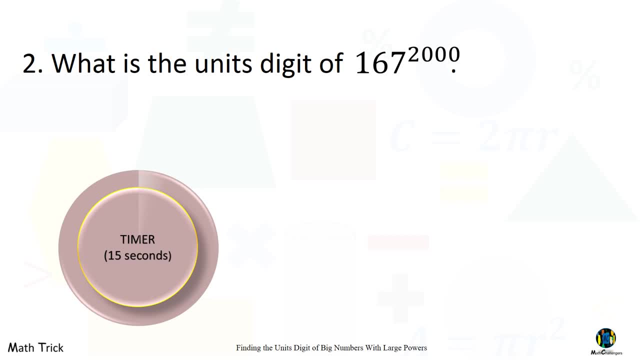 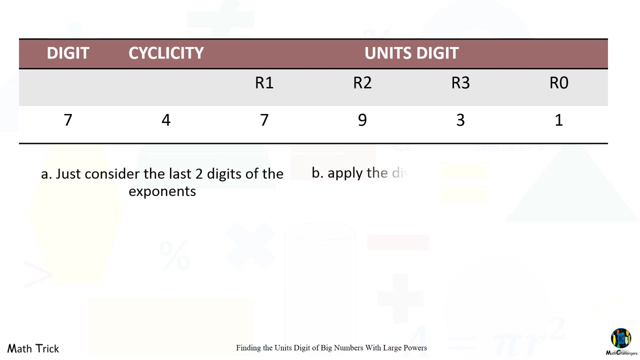 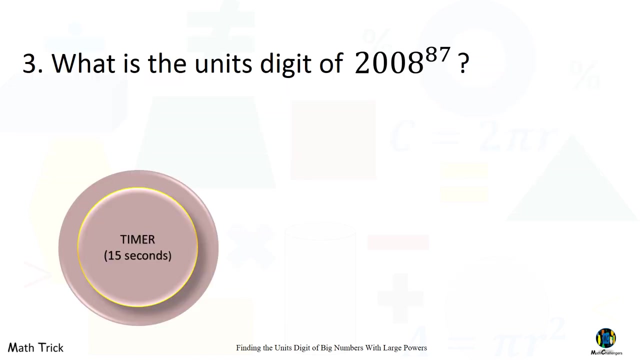 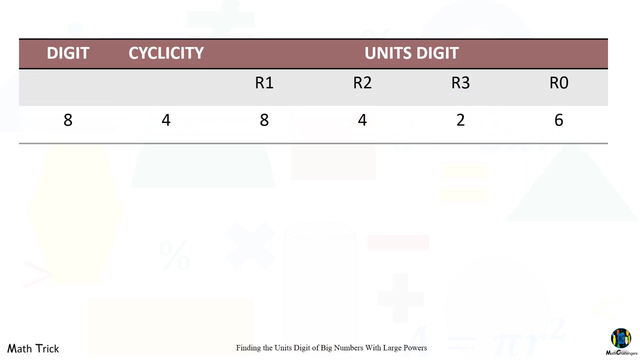 The upper left. second is in the attacks27.. the 2000 power. 3. What is the unit's digit of 2008 raised to the 87th power? 4. What is the unit's digit of 2008 raised to the 87th power? 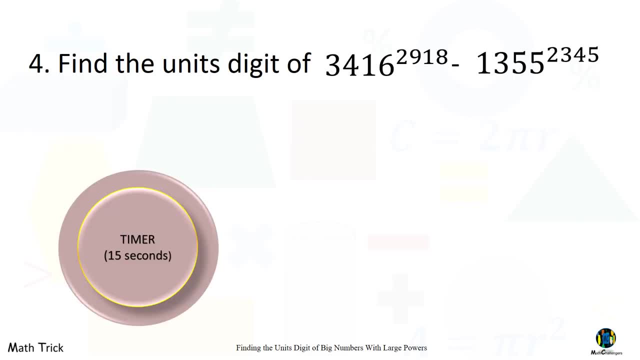 5. What is the unit's digit of 2008 raised to the 87th power? 4. What is the unit's digit of 2008 raised to the 87th power? 3. What is the unit's digit of 2008 raised to the 87th power?